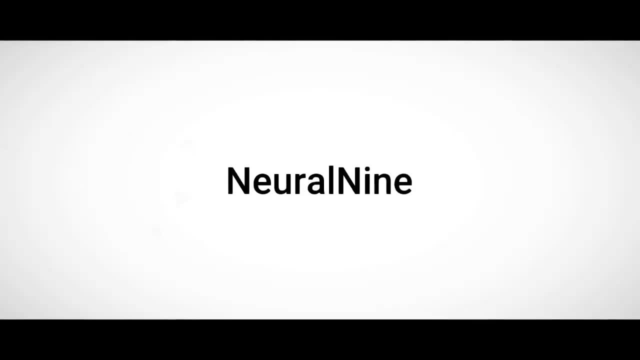 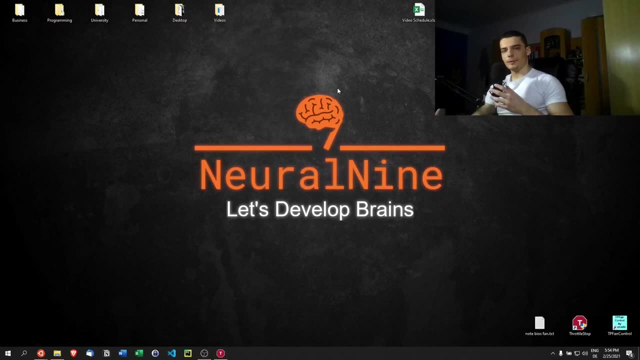 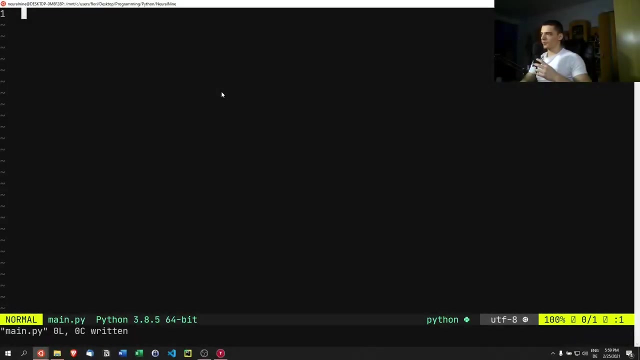 What is going on, guys? welcome back. in today's video, we're going to talk about the composite design pattern, so let us get right into it. All right, so another one of those design patterns now. the composite design pattern is actually quite simple to understand and it's quite intuitive. 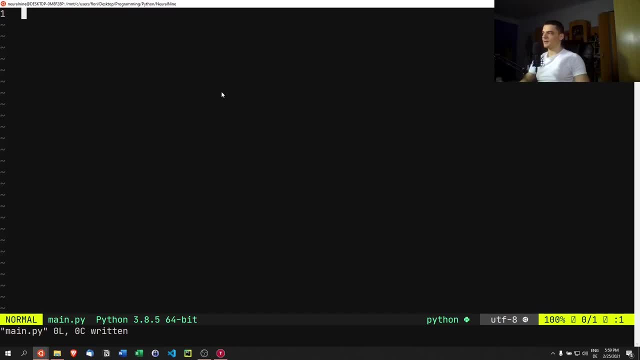 it's not too abstract or too fancy. the idea is very simple and very something that you can grasp with common sense, I would say, and it's basically that we have multiple classes that inherit from the same interface or parent class, and one of those can consist of many of the others. so for 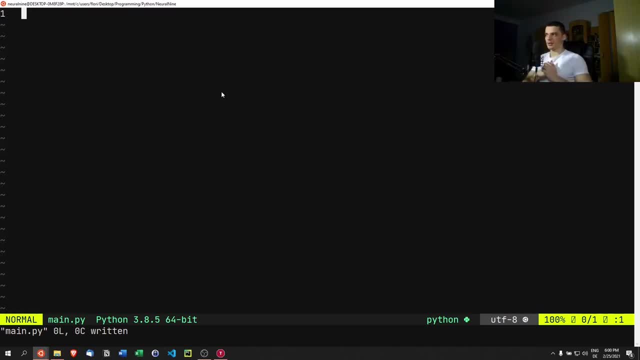 example, if we're talking about regions, we can say one region can consist of many sub regions and those sub regions can consist of other sub regions. and what we're going to do in this video here is we're going to use departments as an example. so we're going to have one parent department one. 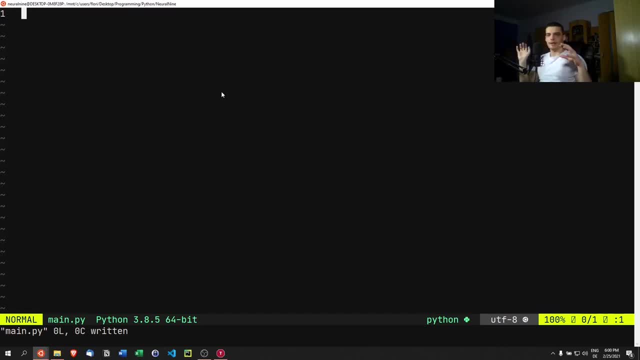 big department which is composed of an accounting department, developer department and so on. and if you want, of course, you can also say that the that the developer department is composed of specific development departments, and so on. so this is the basic idea, and why do we do that? first of all, of course, 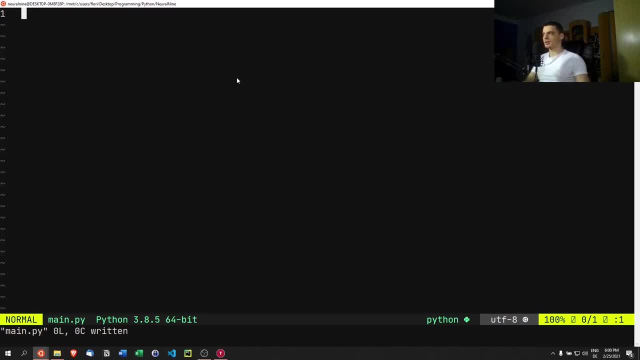 it creates a hierarchy and a tree-like structure, but also it increases the flexibility and it makes the structure easier to use. so you might want to use that in some of your projects. the basic idea is- or actually, let's just start with the basic idea of the basic idea, of the basic idea of the: 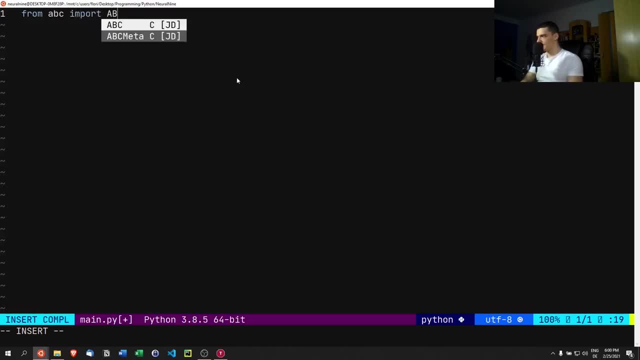 abstract method. and then we're going to- let's just clear the search here- then we're going to have a department interface. so we're going to say class i department, which is going to have the meta class, abc, meta. and here we're going to define an abstract constructor. so we're going to say: 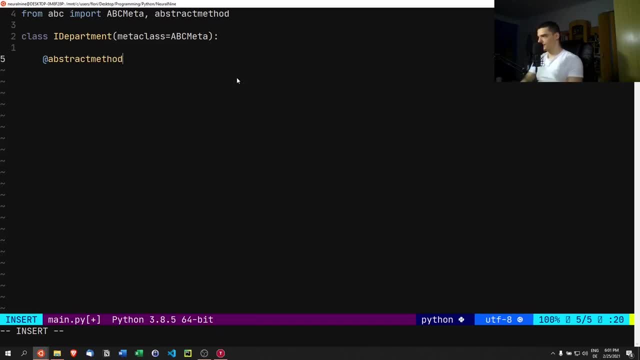 abstract method. abstract- come on- method is going to be the initializer, with self and the number of employees. so this is what we're going to do here. we're going to say a department can have a certain number of employees and, of course, if you have a parent department, 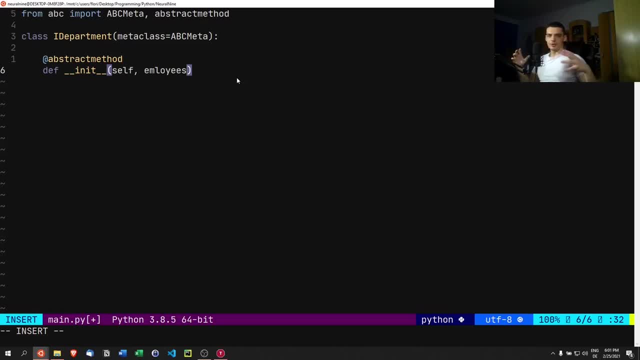 which consists of uh sub-departments. those departments have their employees and then we have a total number of employees there. uh, this is the basic idea here that we're going to try to model and this is something we're going to implement. implement in child class like that. 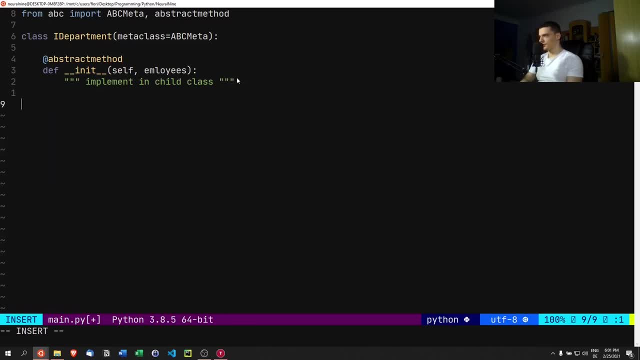 and then we're going to say also an abstract. actually, i think for this we need an abstract static method, so let's import that as well: abstract static method here, abstract static method, and here we're going to have print department, print department, and we're also going to implement this in a child class. 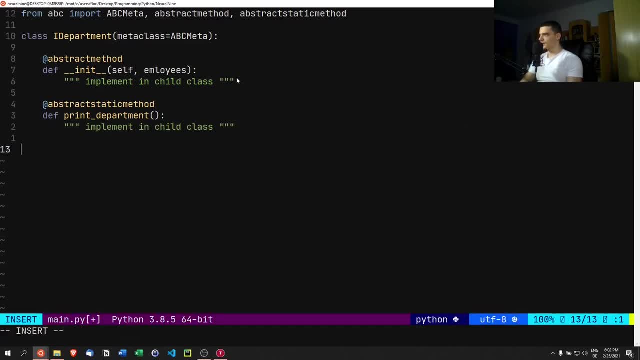 all right, so that's the basic interface. and now we can say, okay, we have an accounting department, so let's say class accounting we're not going to call accounting department, but just accounting is going to inherit from the i department and we're going to override the constructor here. so 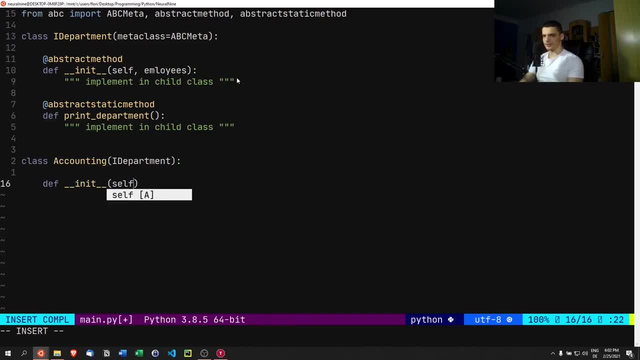 we're going to say: init is just going to be self and employees and we're going to say: selfemployees equals employees. that, um, we are missing a p here. so employees, and we're missing it here as well. so let's add that as well: employees. 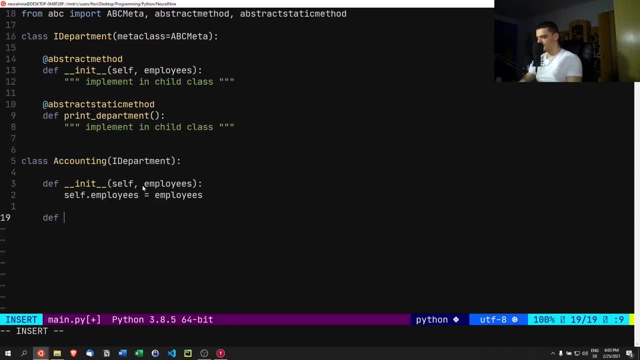 uh, there you go, and then we're going to have the print method. so we're going to say dev, print department, and i think we need to pass a self object here, or do we? yeah, we need to pass a self object here, and then we're going to say print. 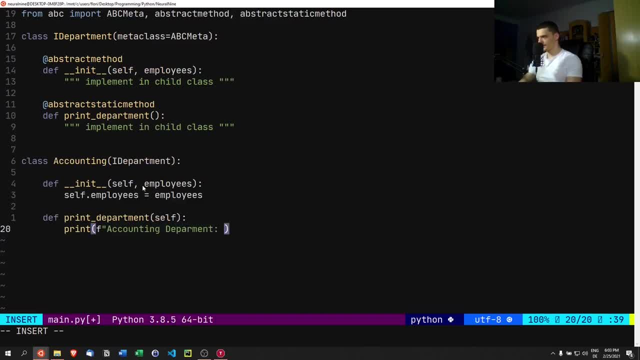 accounting department and we can print the amount of employees in this particular department. so we're not going to divide this one into sub apartments. this is just going to be- uh, you could, you could say a leaf department, since it's at the leaves of a tree, so we don't have any childs here anymore. uh, and we're going to have another one of those. 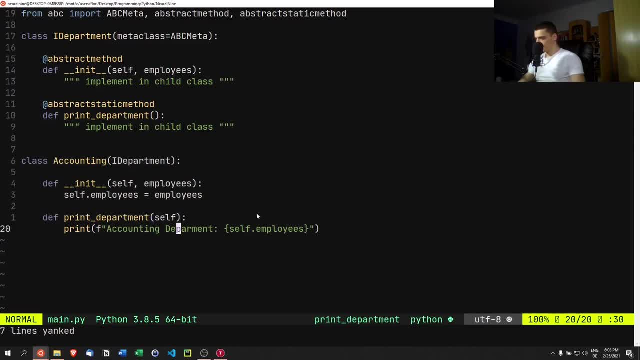 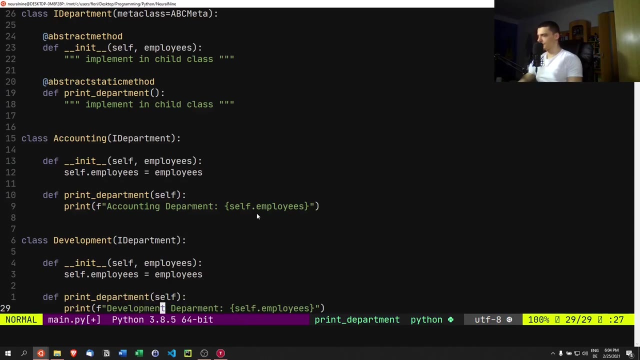 so we're going to just copy all of this here and we're going to paste this here and we're going to rename it to development, for example, and then here we're just going to change the test to development text to development department, and this is the. 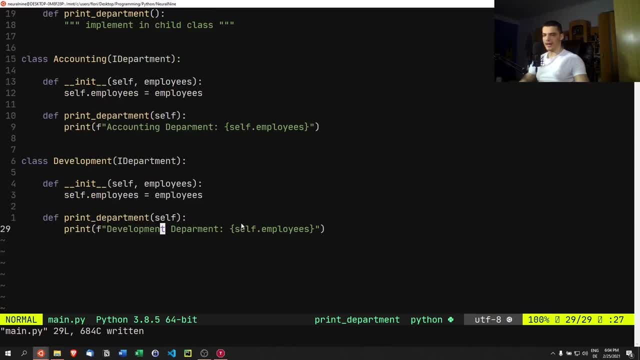 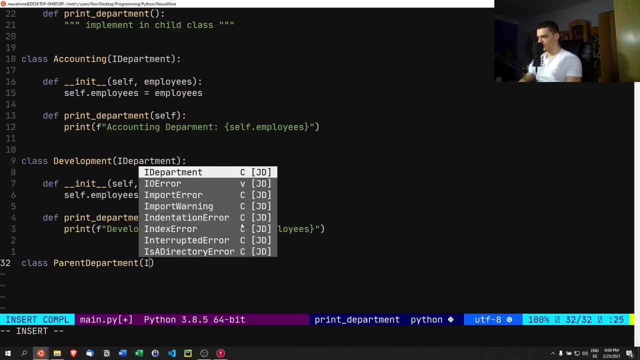 basic, those are the basic two leaf departments you could say. and then we have one parent department. so now we're going to say class parent department, which is also an i department, and here we're going to do it a little bit differently. so here we're going to have 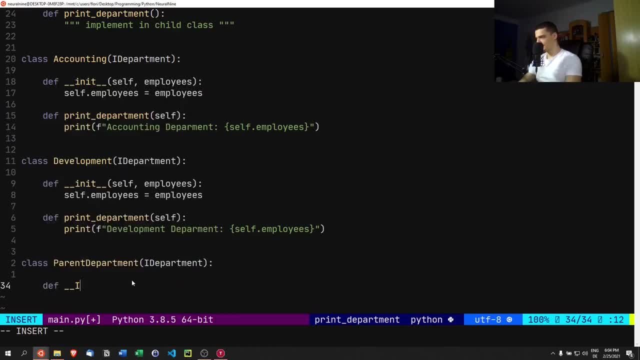 basic constructor again, but we're going to add some functionality here. so we're going to say def init and again, self employees, because the parent department on its own, without looking at the child departments, is also going to have, uh, some employees, and we're going to say the 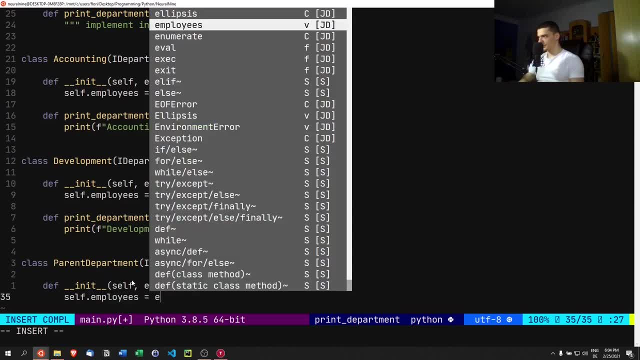 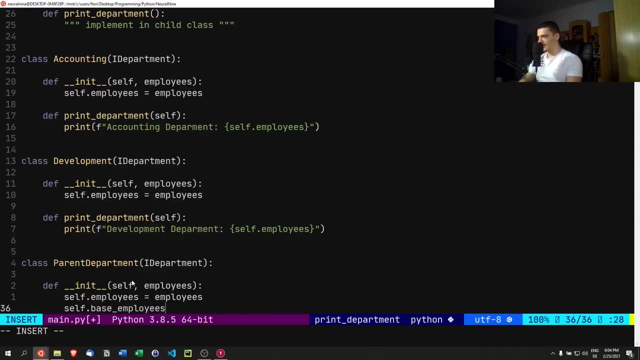 employees are going to be starting at that number because those are the base employees. but then, in order to not lose track of that number, we're also going to say: we have the base employees and we're not going to change that number, so that we know how many of those employees are. 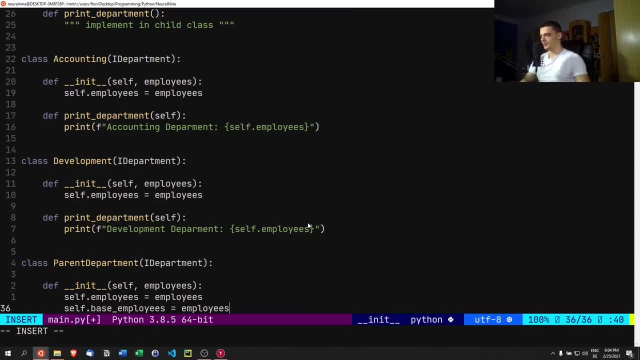 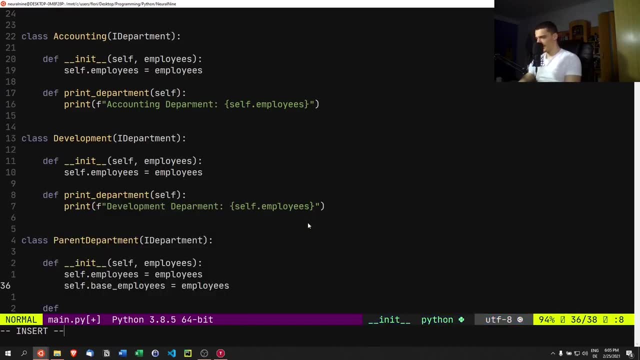 actually part of the parent department without being part of the child departments, and then we're going to have the print method, or actually we need to add one more thing, because we need to be able to add departments to the parent department. so we're going to say self dot sub. 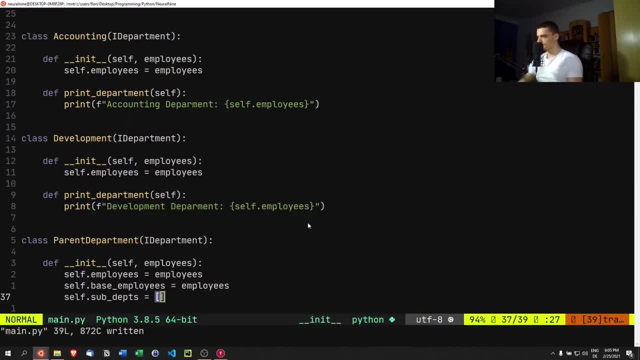 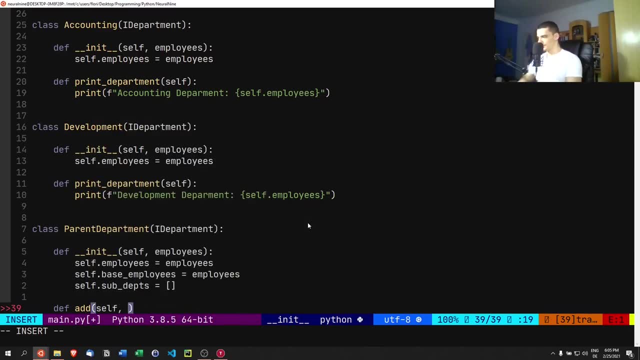 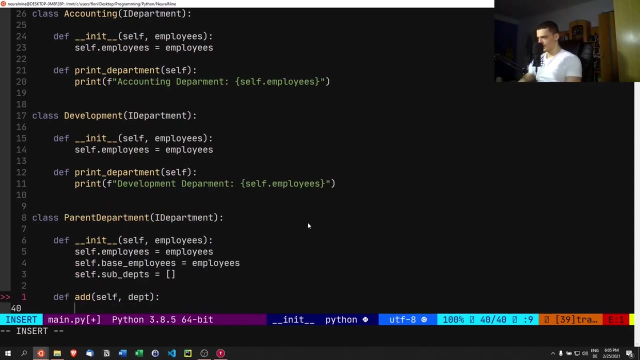 depths is an empty list and then we're going to add an add method here. so we're going to add a department to this list. so we're going to take self and a specific department into this list here and we're going to just say self, dot, sub departments. 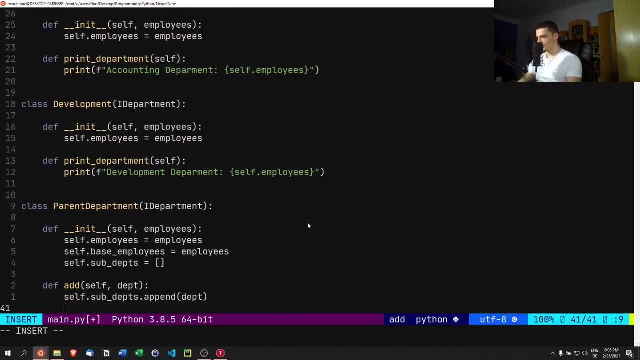 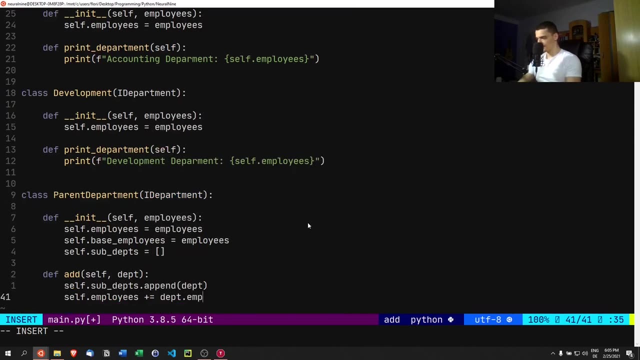 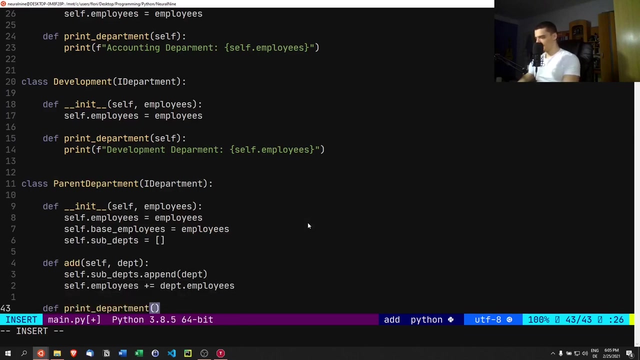 dot append department, and we're going to increase the number of employees, not the base employees, but the employees at all in general. we're going to increase that by the amount of employees in this um, in this department, like that, and then we're going to have the print method here, which is going to be the print department method itself. and now 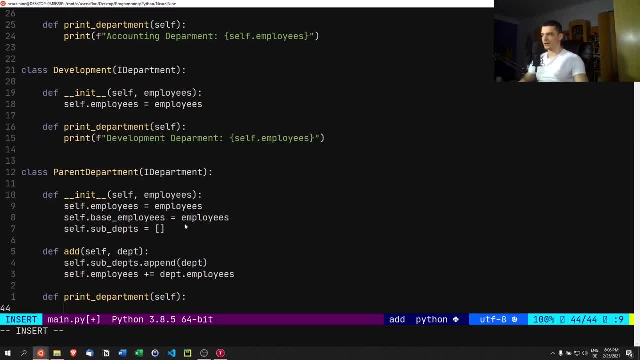 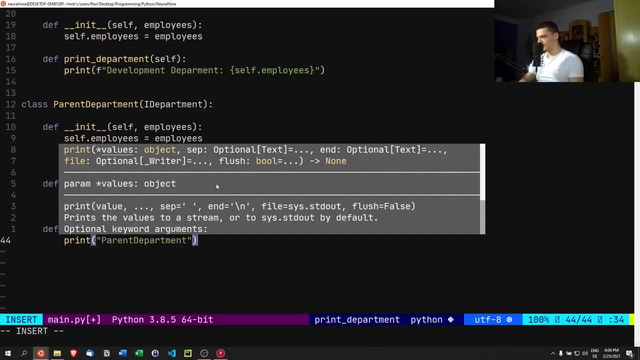 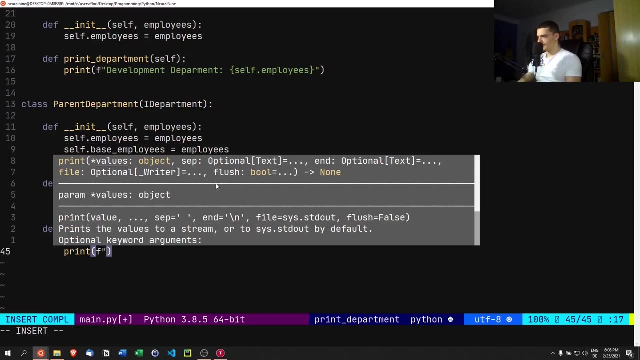 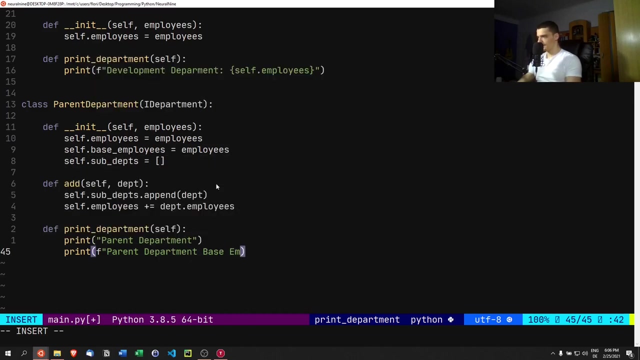 we're going to print not only the information about the parent department in and of itself, but also about the child department. so we're going to say print parent department, for example- actually maybe use a space here, parent department- and then print: um, parent department base employees is going to be just self dot base employees, like that- and then we're going to say for 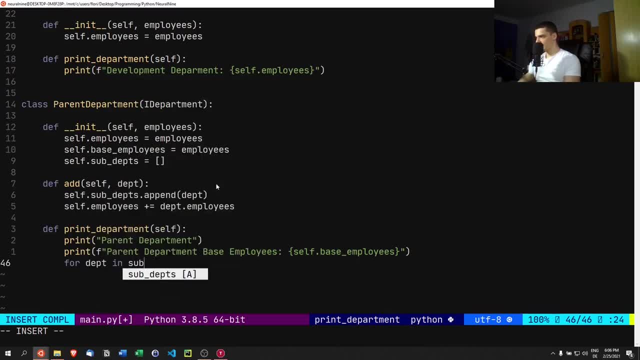 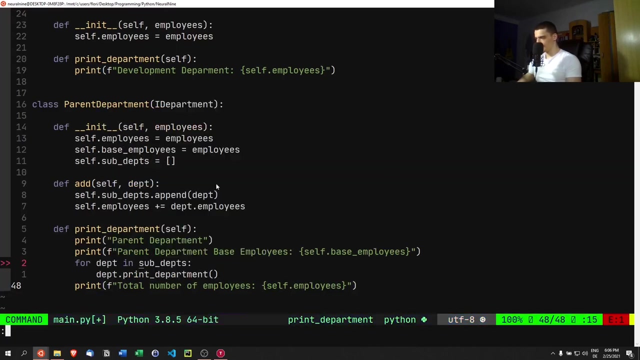 every department, in sub departments, we're going to say department print department, so that we get this information as well, and we're going to print total number of employees is going to be self dot employees employees, because this number is constantly being updated and here we're going to add an f. 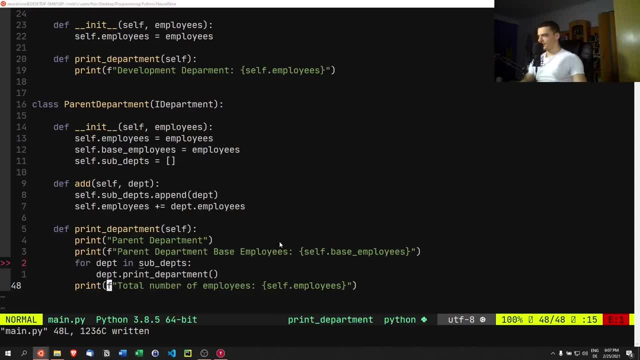 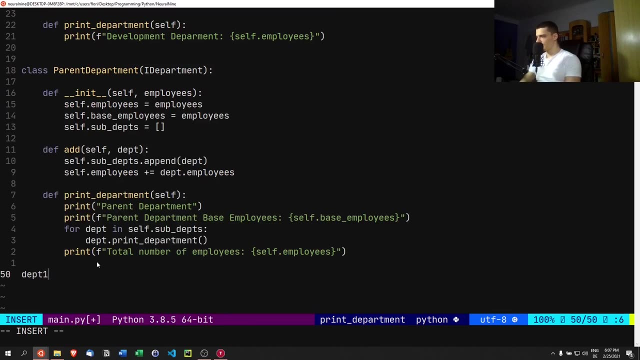 for the f string, and then we can actually: sorry, then we're actually done. what do we have here? sub depth's? oh self dot sub depth. sorry, then, we're actually done, because now we can go ahead and use this, but just saying, department one is going to be the accounting department, with 200 employees, for example, and department two is: 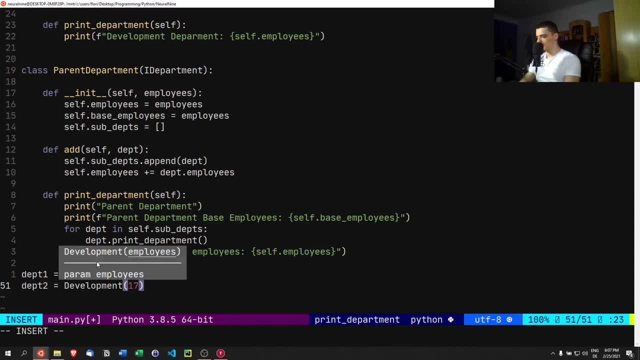 going to be the developer or the development department, with 170 employees here, and then we're going to have the parent department, which is going to be just a parent department with a base employee amount of 30, for example, just some administrative tasks there, and then we can add to. 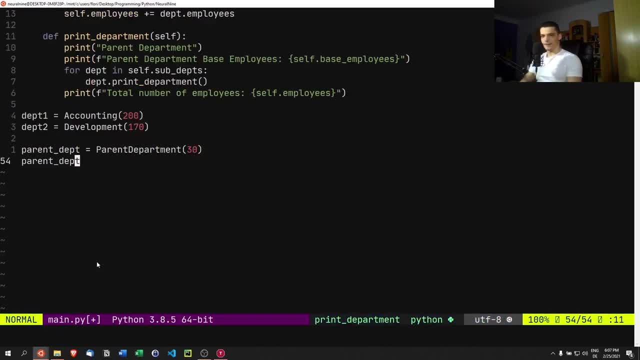 this parent department. let me just center this here. we can add to this parent department department one and department two, and then we can go ahead and print everything. so parent department, print department. there you go. that's it. take a look at the code again. let me just make sure that. 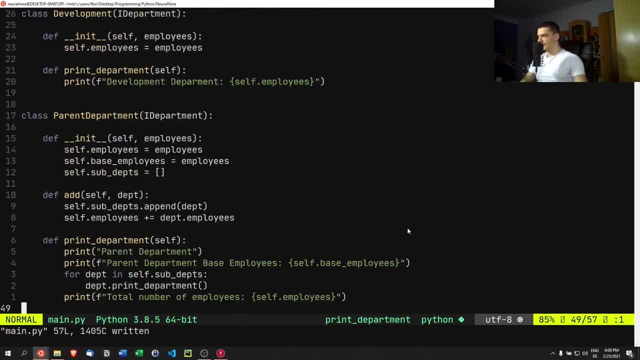 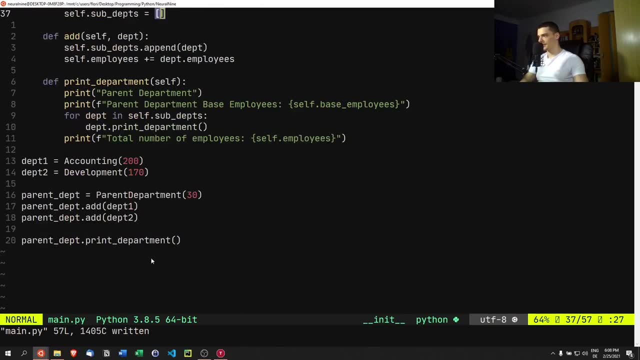 i'm not blocking everything, no, i'm small enough. so this is the code again. we just have, um, the interface and two basic- uh leaf- departments, you could say, and then a parent department which adds those departments together. so a very simple design pattern. let's take a look at it. terminal.